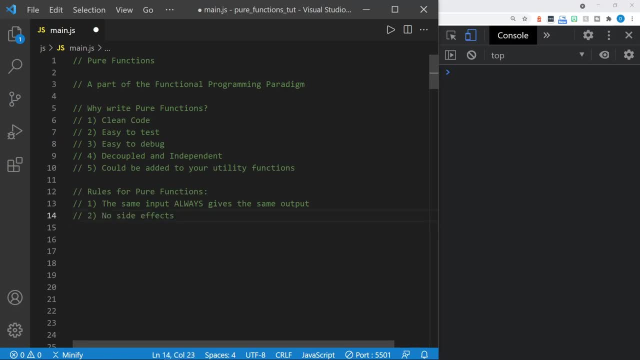 The second rule is there should be no side effects, and we'll talk about side effects in a minute, but first let's break the rule one down with some examples. Okay, the first rule of pure functions: the same input always gives the same output. So let's look at this function just called add. 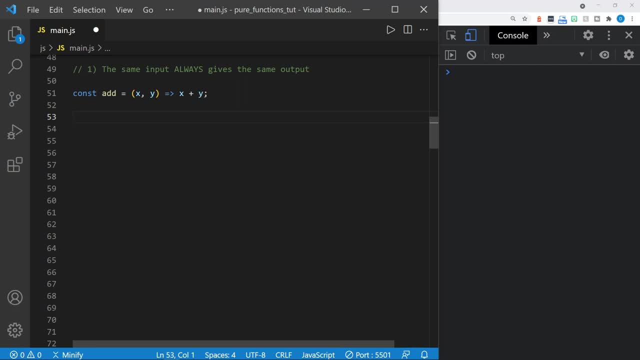 a very simple function that accepts two arguments, x and y, and it adds those together. Now if we log this to the console and we'll call the add function with two and three, you can see we get five, and it should always be five and there's no reason that this wouldn't be. 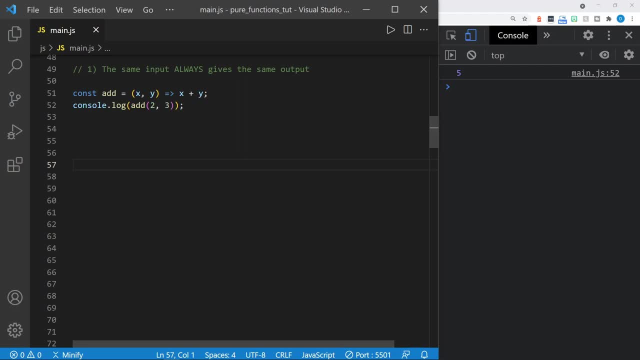 and we're passing in primitives that primitive data, and so it passes values. so we're not modifying any data, which will be side effects that we talk about in a moment. So this is a pure function add, and mathematics is an easy way to think about this, because 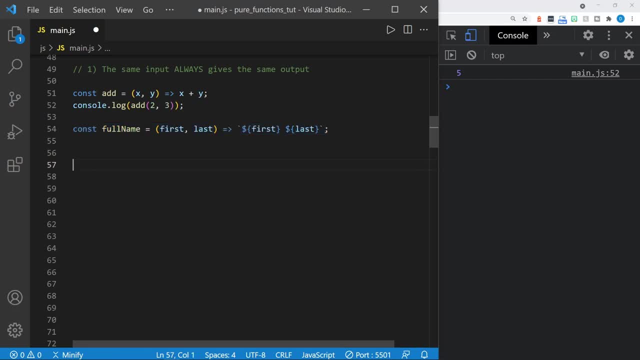 it provides pure functions like this. Another function would be full name. This is another simple example here, and I'm providing two arguments, first and last. and then we're using a template literal string to concatenate those into the full name. Now, when we go ahead and 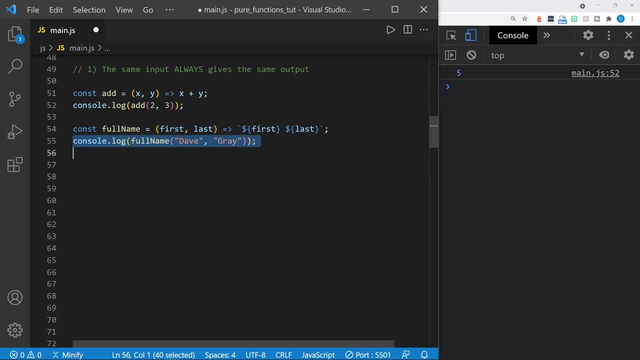 log that to the console and we call it with the parameters of my first and last name. you can see we get what's expected and that's my full name, Dave Gray, and it would always return that value. So these are predictable. the same input always returns the same value. 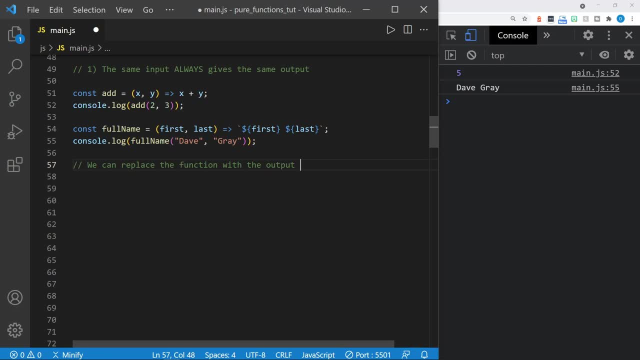 gives the same output and we can replace the function with the output itself, and this is called referential transparency, and it's very important for pure functions. that's what makes these easy to test and easy to debug. a pure function should have at least one parameter. let's call this rule 1a. 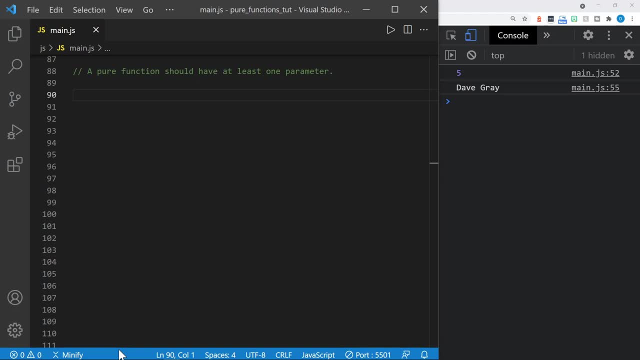 because it's not usually listed as a rule of pure functions. but I will show you why you want to consider this. otherwise it's really the same as just a constant, because a pure function can only work with the input that it receives. so consider this function first name and it just simply returns my first. 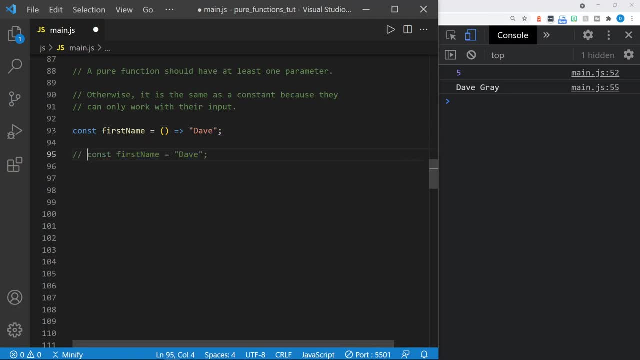 name, but we might as well just define that as a constant say: const. first name equals Dave, because it provides the same thing. a pure function should not work with any data that is not provided as an input parameter really. so this would be the same, and so you can see why a pure function should. 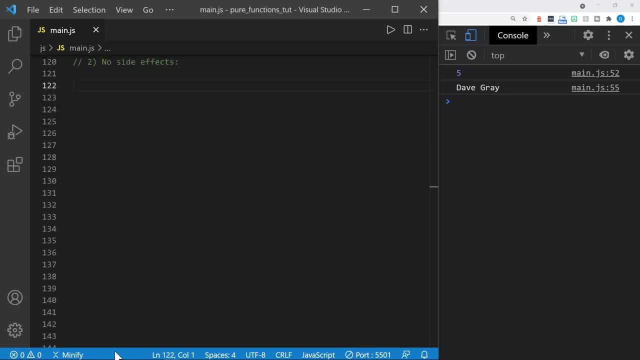 have at least one parameter. okay, rule number two for pure functions, and that is no side effects. this could take just a little longer to understand all the possibilities of side effects, so let's look at some examples. and this also means accessing the scope outside. the function makes it impure. so here's an. 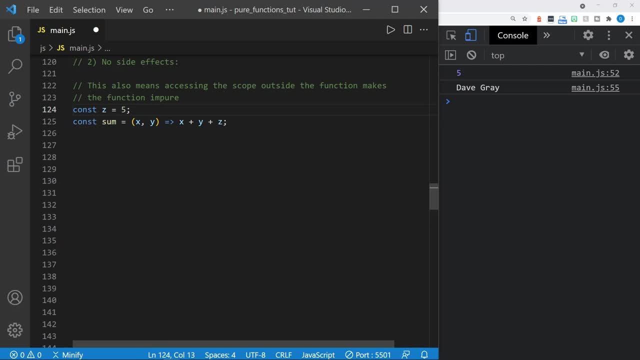 example, where I define Z equal to 5 outside the function sum, but then notice how I reff Z inside the function. this is totally possible in Javascript. we're just accessing the global scope here and in a function you can access the lexical scope that is outside of the function. 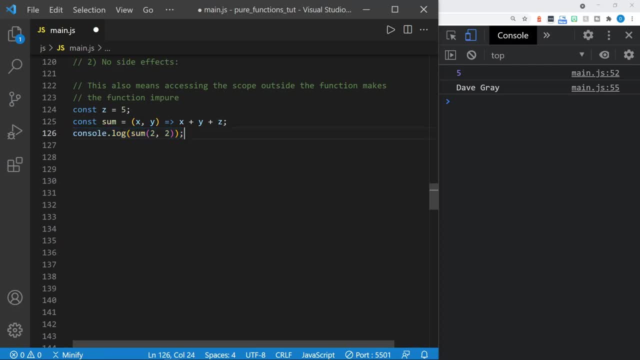 but this makes it impure. so when we go ahead and call this function sum with 2 and 2 for the parameters X and Y and we save the file, we get 9, because the function still has the importa function just doesn't support it. and it can't work because view. 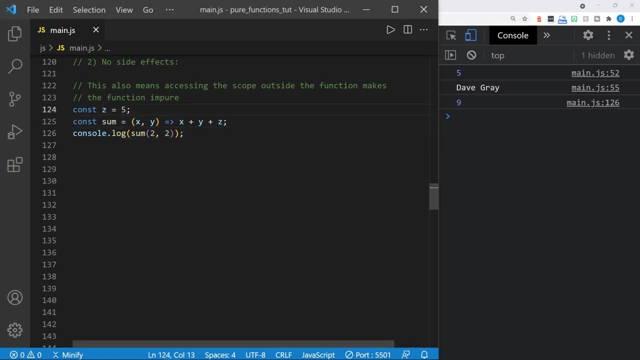 has access to the value of z because it's inside the lexical scope. it's actually outside the function, but that makes this function impure. so pure functions cannot access a database, an api, file system, storage, other parts of the network etc. and they can also not modify the dom. 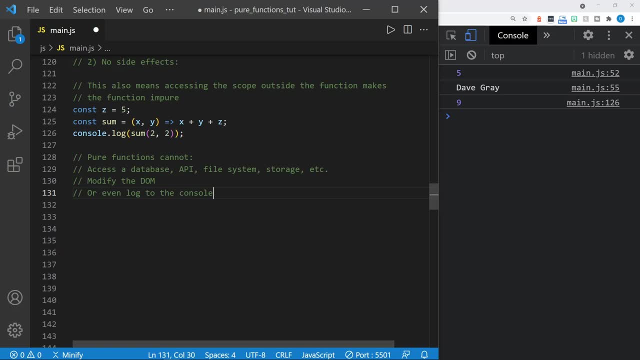 and they can't even really log to the console because that's doing something outside of the function itself. and so, that said, clearly impure functions are necessary because they're hard, but they're harder to test and debug. but that doesn't mean impure functions are bad. clearly we need to. 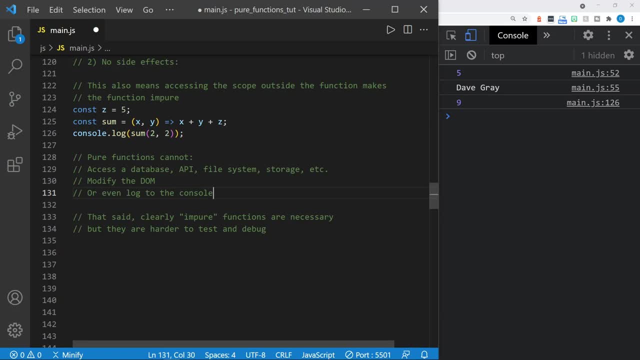 modify the dom at times and clearly we need to access a database or an api or the file system. so impure functions aren't bad, they're just harder to test and debug. and from that we need to say: no input state can be modified. you, we're writing a pure function and that means no data should be mutated. and that also means you. 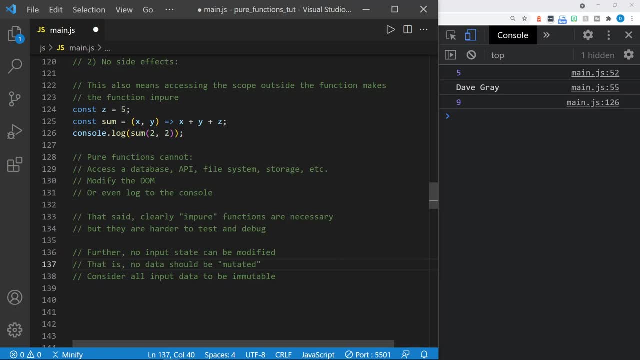 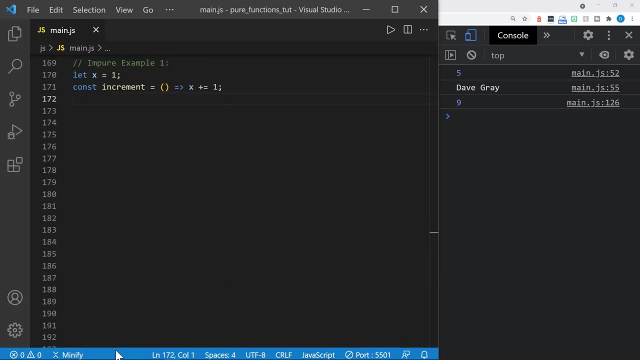 should consider all the input data to the function to be immutable when you're writing a pure function. let's look at some examples. let's look at this first example of an impure function, where i'm defining the variable x equal to one, and then i'm incrementing the variable and by calling the 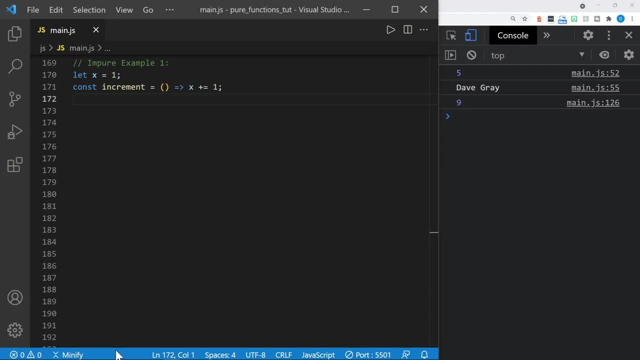 function increment, but this breaks all the rules of pure functions. let's go ahead and call increment and then we'll log x to the console and you can see, after we call increment, we are logging two. and then we check the value of x on the next line and the value is two. so we mutated the state of the x variable. it's now equal to two. 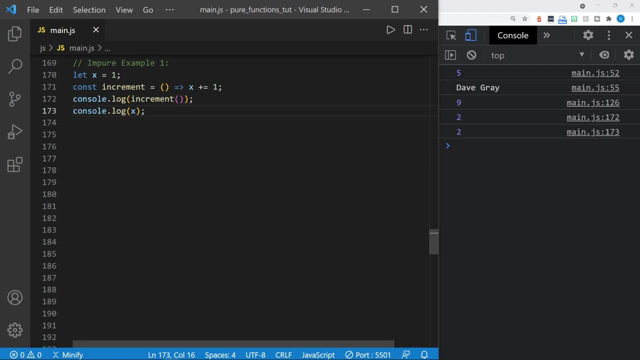 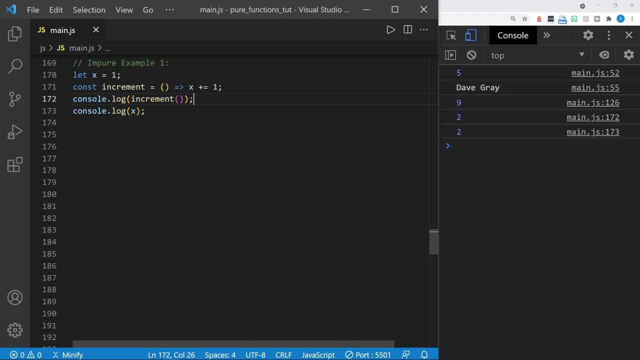 actual variable x. we don't want to mutate x, but we do want to return a new value. so this is an impure function. it breaks both rules. there we we don't pass in x, and then we also mutate the value of x. next example: we've got my array equal to an array that just has the numbers. 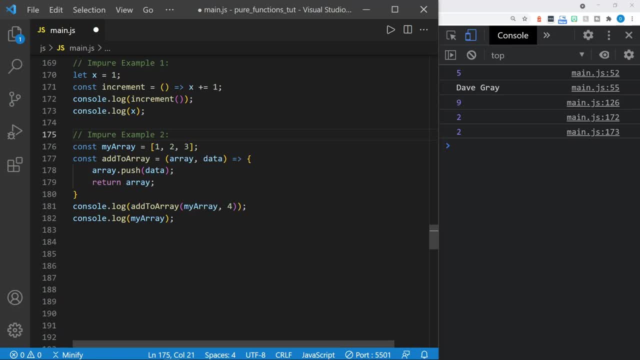 one, two, three and we've gotten a. we have a function called add to array and this function receives an array and data as parameters, as arguments, and now we reference the array and we push the data to the array, then we return the array and now we'll call the. 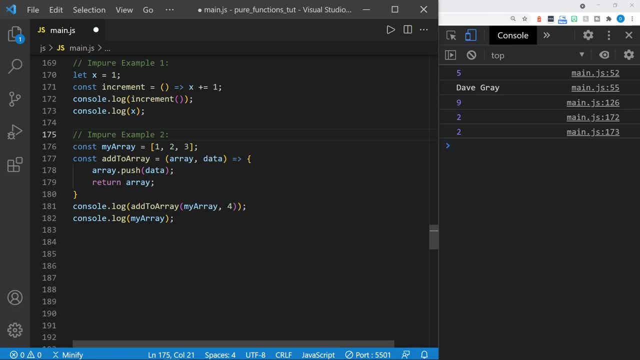 add to array function and pass in my array and a new number, the number four, and then we'll check the value of the original array and see what elements are in that. so if we save this and look over here in the console, you can see that we returned an array with one, two, three, four. but 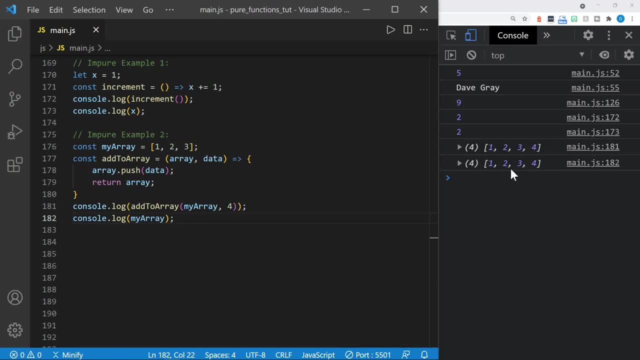 unfortunately, the original array, my array, was mutated and it also now has a fourth element, and you don't want to do that. now this is an array- is structural data versus primitive data from our first example. but you don't want to mutate the structural data either, and we did that. so this is. 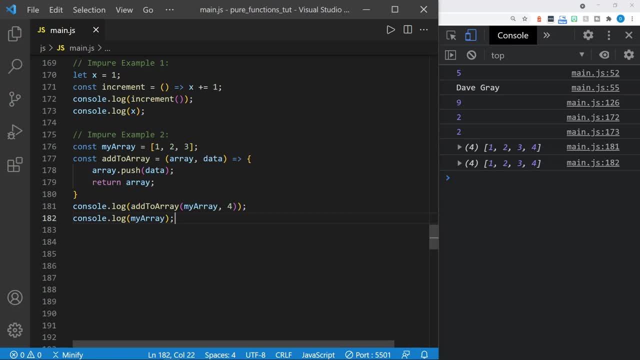 also an impure function. now let's look at how we can refactor these functions as pure functions. in our first refactoring example, we are now using a function called pure increment instead of increment, so we have one parameter, as we would expect for a pure function to receive at least one parameter. 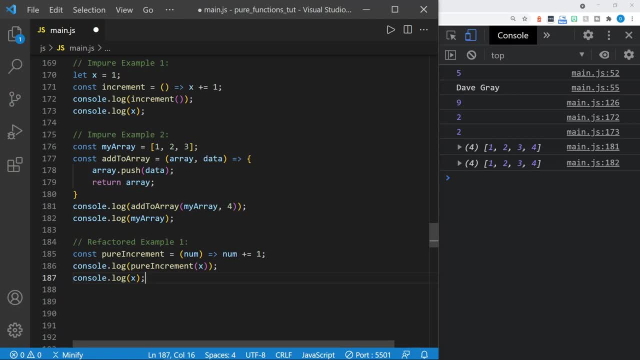 and that parameter is a number, and then we increment the number, but we're not changing the value of what is actually sent into the function. so we'll call pure increment on X and then we'll go ahead and log X to the console. you can see the result of pure increment X on line 186. 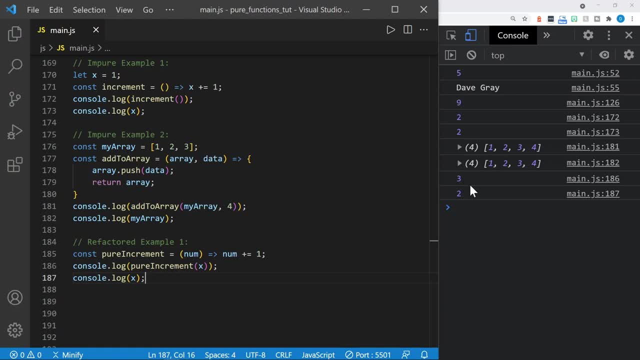 is 3, but once we check the value of X itself, X is still 2, and this is primitive data. we've got a variable with the value of 2, and primitive data passes values, and so that is why this works, and if you're not familiar with those, I'm going to reference a video and link to it in the 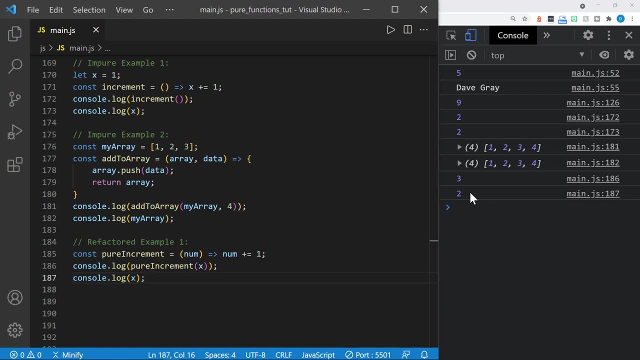 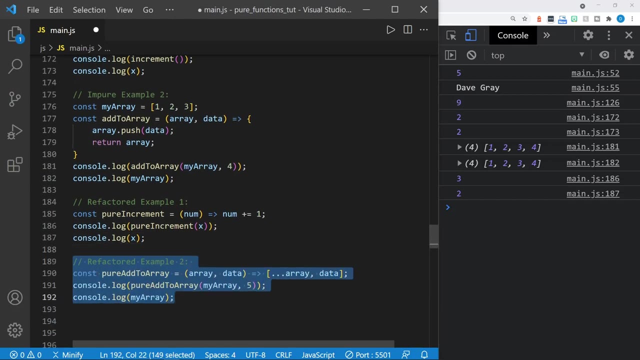 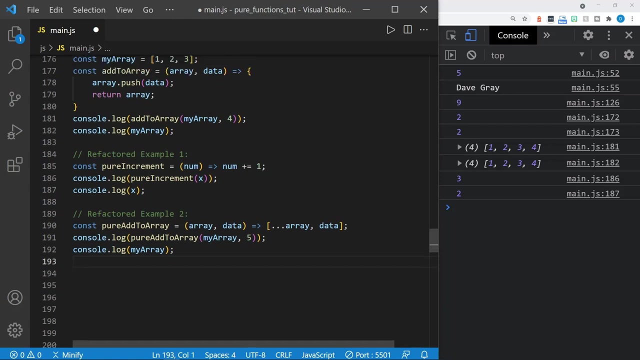 description as well, where I really compare a shallow copy and a deep copy. however, I discuss primitive and structural data in that video tutorial as well. okay, let's look at our second refactored example, and in this refactored example we have a function called pure add to array. I guess I'll scroll back down a little so you can see the original there. 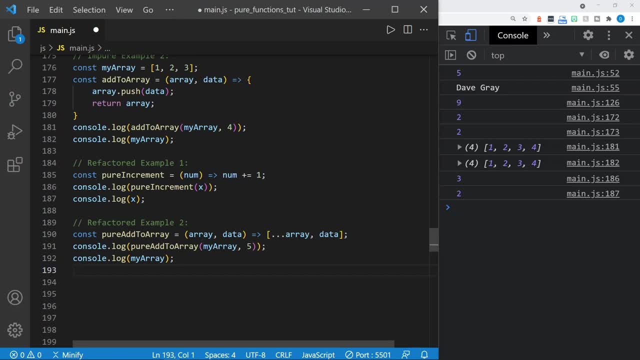 and so the original is at the top. but now we have pure add to array. that receives an array and it receives the data, and then we just return a new array using the spread operator and then we add in the data. so it's a new element in this array, but this is a new array. so once we call this on the next line, 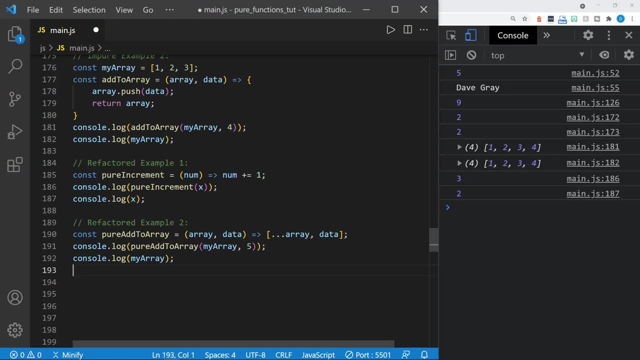 with my array and the number five. we'll see what we get there and then we'll compare by logging my array to the console and if we save this you can see the pure add to array returns a new array with five, but the original my array still only has one, two, three and four. so we did not mutate the data. so 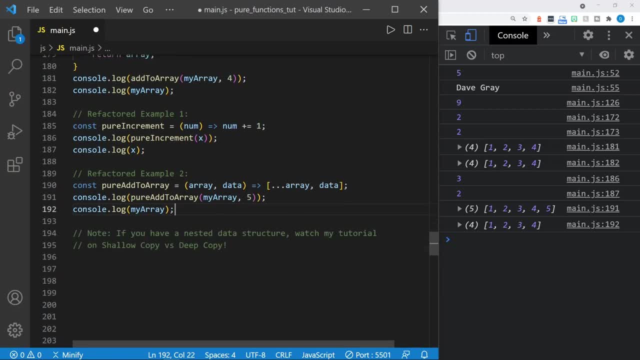 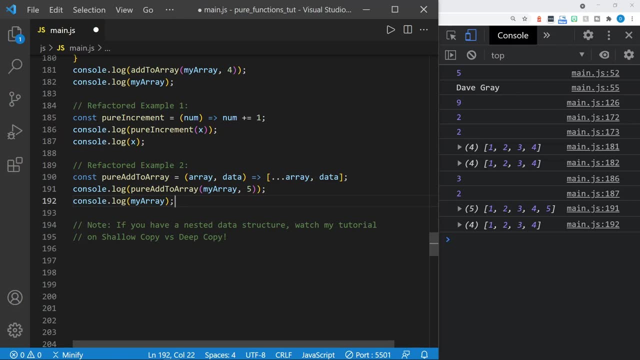 this is another example of a pure function. so note if you did miss my previous tutorial on shallow copy versus deep copy. you'll want to check that out because the refactored example two above will not work if it is a nested data structure. if the original array we're passing in has nested data, you 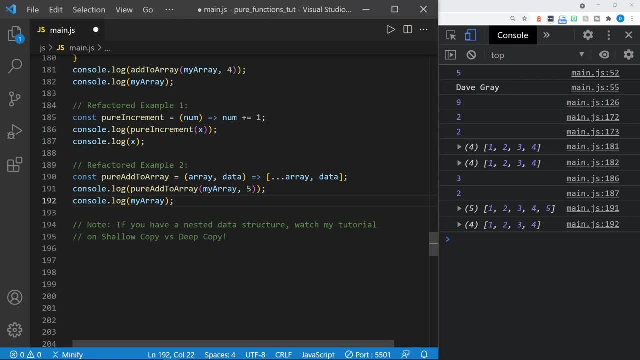 need to make a deep copy- and I show you how to do that in that tutorial that I will show up above right now- and, of course, I'm going to link to it in the description as well- and then also notice how pure functions always return something. this isn't one of the rules that is always listed for pure functions. however, if 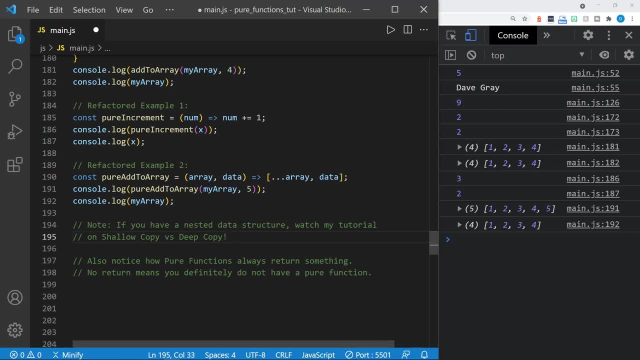 you're not returning something, you definitely do not have a pure function. so that is one easy way to tell if you have a pure function or not. or it doesn't necessarily mean you have a pure function when you return something, but if you're not returning something, you definitely do not have. 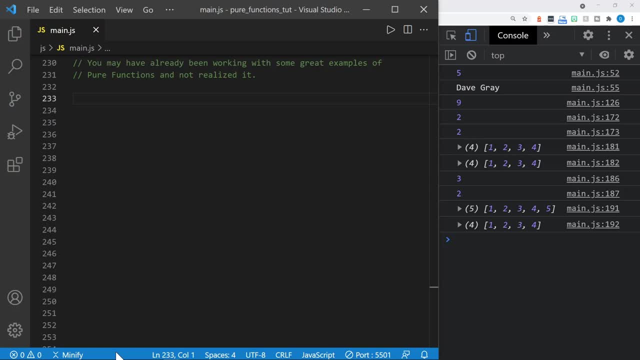 a pure function. you may have already been working with some great examples of pure functions and not realized it, so some common higher order functions are pure functions, and so I'm going to start out with this array that just is called one to five, and it has the numbers one through five and then 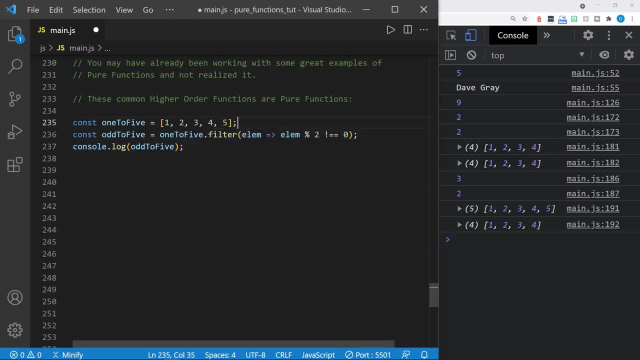 I'm going to define odd to five and use one to five with the answer method on the array and you can see that I plan on returning the odd numbers. so if I go ahead and save this now, odd to five just returned one, three and five. that's a new array with just the 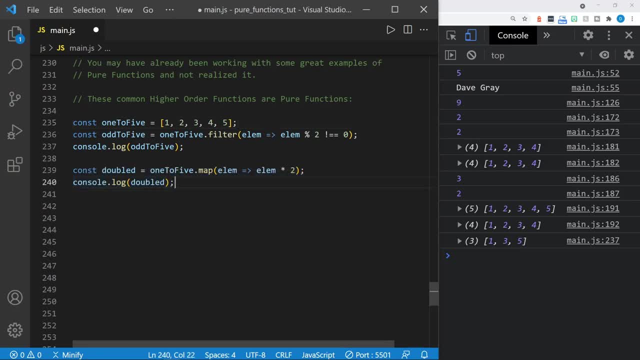 odd numbers. and now let's look at another example. I'm defining doubled and I'm calling the map method on my one to five array and now I'm multiplying each element in one to five by two, and then I'm going to log doubled And when I save this I've got 2,, 4,, 6,, 8, and 10.. So 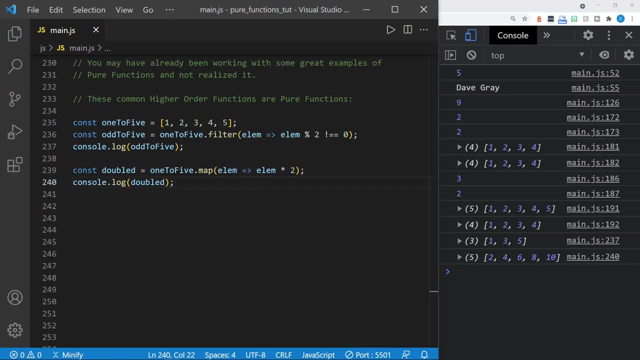 the numbers 1 through 5 have each been doubled and they're in a new array. And then, once again, I'm going to define summed and I'm going to call reduce on 1 to 5.. Now reduce receives not just the element of the array but also an accumulator, And then we add the accumulator. 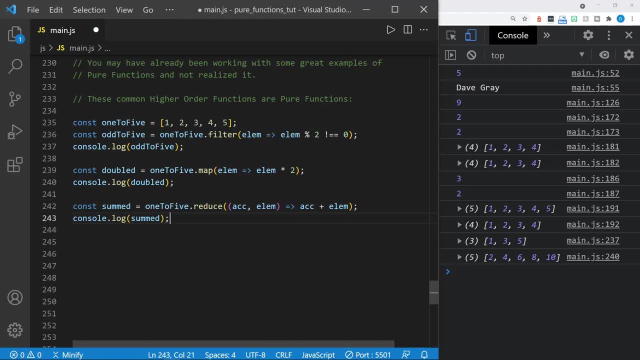 and each element of the array, so it totals them up And then I'm going to log summed to the console as well And you can see I get the number 15.. So if we come back and just log the original 1 to 5, 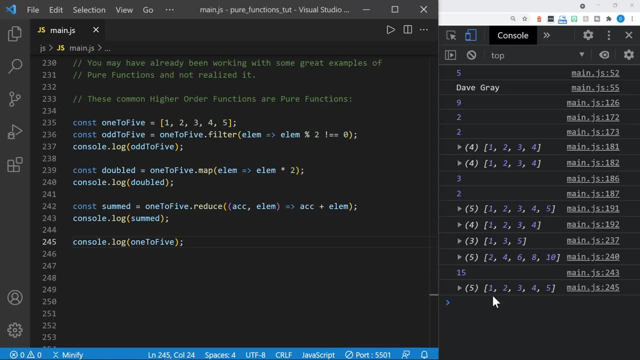 array and I save that. you can see it is still the original array, 1 through 5.. So all of these higher order functions that you may have already been using all follow those rules of pure functions. They're returning a new value or a new array, They're not modifying the original, And so that's. 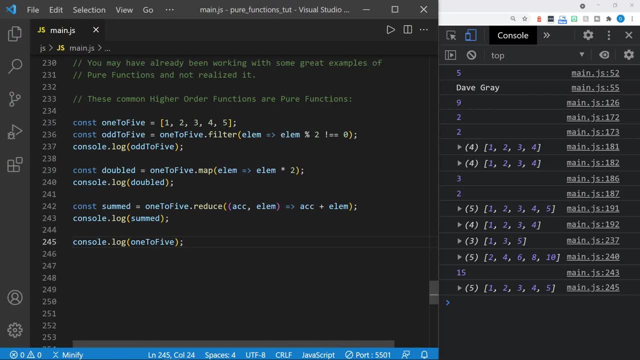 kind of what pure functions are all about. And if you're not familiar with these higher order functions, I do have a tutorial for those as well that I shall link to above and put a link in the description below. Just a quick review of the rules for pure functions before we finish, And the first: 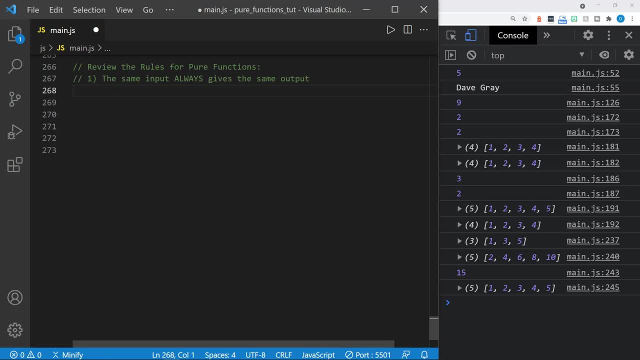 one is the same: input always gives the same output. That is, you should be able to replace the function with the output And your application would still work, And that is referential transparency. And then no side effects, which means no mutations. You do not mutate the global state, You do not even really access. 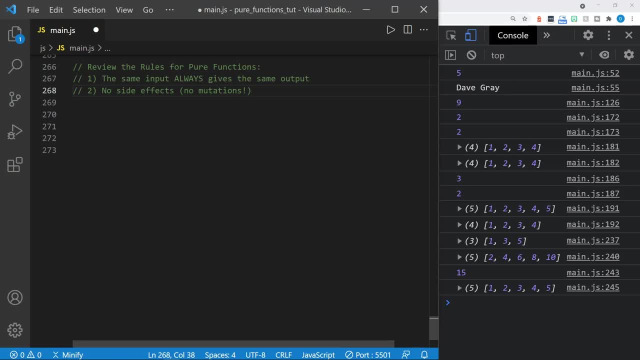 anything outside of the function And the input parameters you give to the function should not be mutated in any way. So if you pass in a new object or array, you shouldI mean if you pass in an object or array, you should be returning a new object or array to the function. Another that I have to report to the 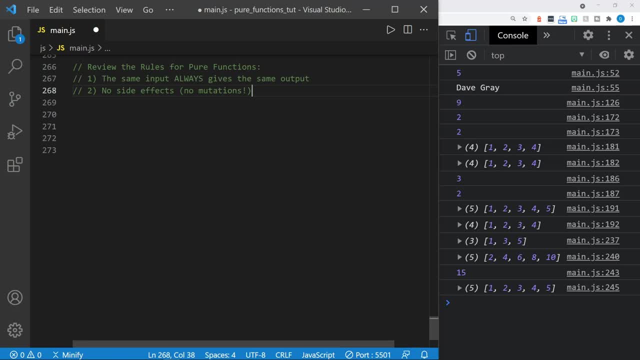 object or array if you're doing anything to it, because you should not modify those structural data types that you pass in or even just any variable value you pass in. You should always return something new. Do not mutate the inputs And overall, the goal when you're working with. 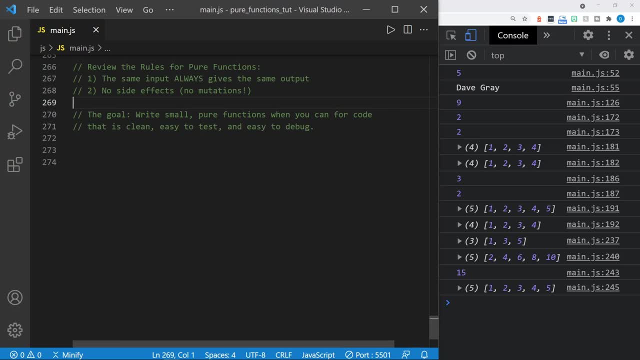 pure functions and kind of thinking along. this functional programming mindset is to write small, pure functions And when you can do that, it helps your code be clean, It's easy to test and easy to debug. So, while you don't have to adopt every aspect of functional programming- and, believe me,